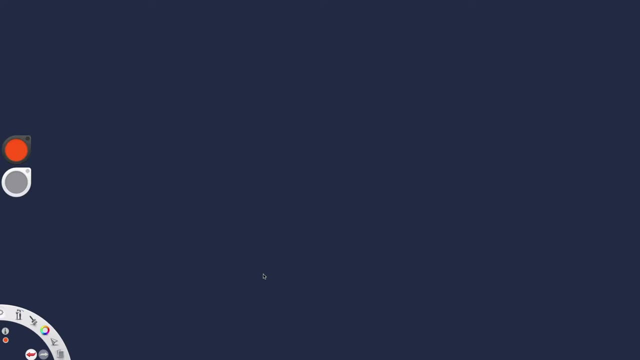 I wouldn't think. but you know, the basic fundamentals are probably certainly could be there, And so let's cover that. Compound names and we'll look at a couple of different things that you know might show up here. The most basic, simple naming convention of a straight 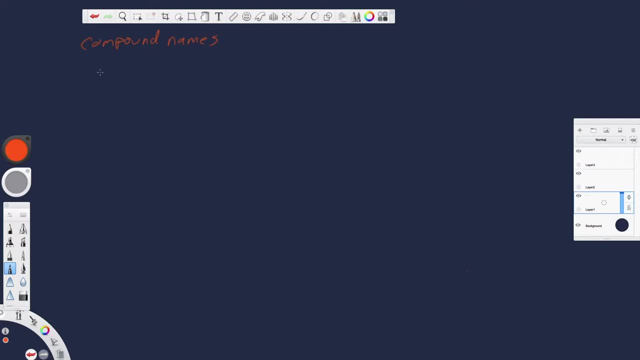 chain would be probably, you know, a straight chain of a straight chain, of a straight chain of a unit. Anyways, here we go. A state of the organic compound to complete its oxidation shell, We gonna what we're going to call gridation. all right, what do we? what we're going to call a gridation is also for the expушки kin de and the first thing you start with. so if we look at just a straight organic compound, And remember, every carbon atom is going to have four bonds of some sort. right, because carbon needs for to complete its oxidation shell. 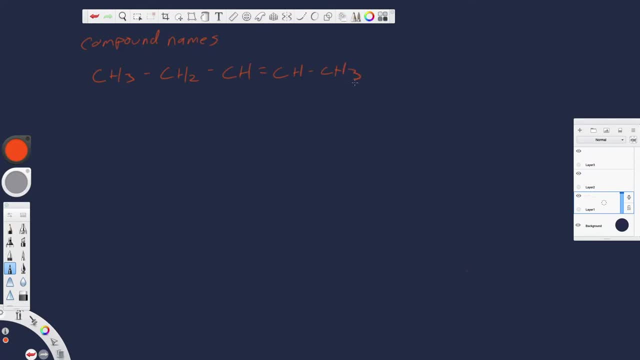 and so all of these should have. you know, here we got three hydrogens in a bond, right? two hydrogens, or i mean a hydrogen bond, and two double bond here, right, and by the way, it's obviously it's a double bond, and so to name this, this one's pretty simple. this is about as easy as it's. 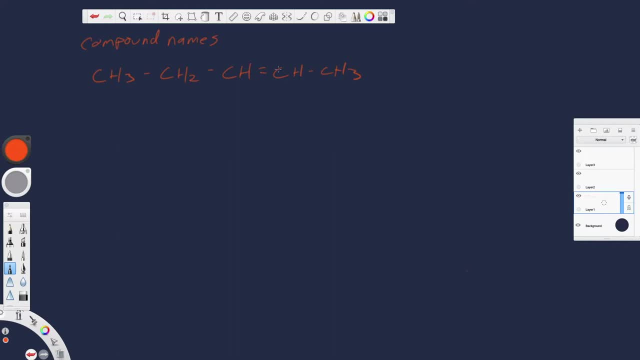 going to get. you have a straight chain here. the only little bit of a loophole or not loophole- the curveball i guess would be right here with the double chain or the double bond. i mean, excuse me. so that's something to watch out for, and you're always going to name your compound from the side. 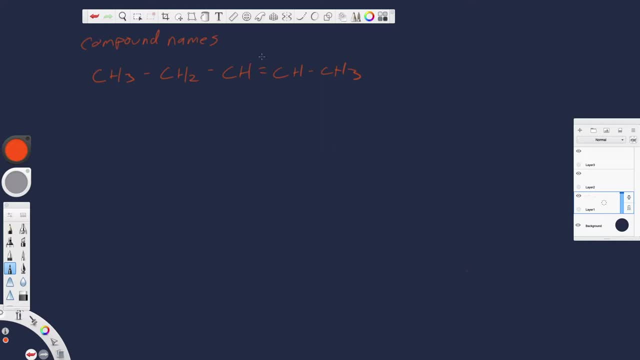 of- and you know things can get more complicated, of course, but in the simpler systems you're going to be naming it from the side with a double or triple bond, or if you have a branch and no other double bonds. so in this case we have, this would be methane. 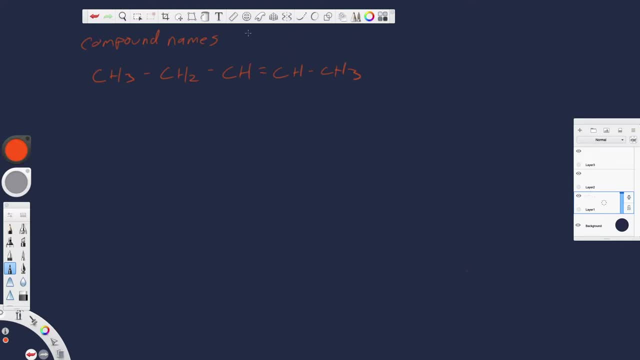 this would be ethane, this would be propane, this would be butane, this would be pentane. so five is going to be pentane if there were no double bonds. but since we have a double bond we are going to have, we would write this as pent to ene, right, if it was. if there were no double bonds, it'd be. 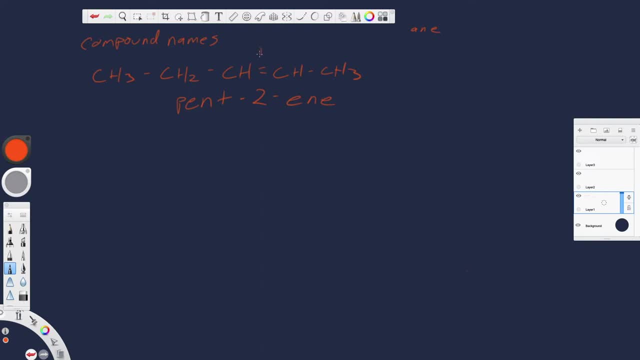 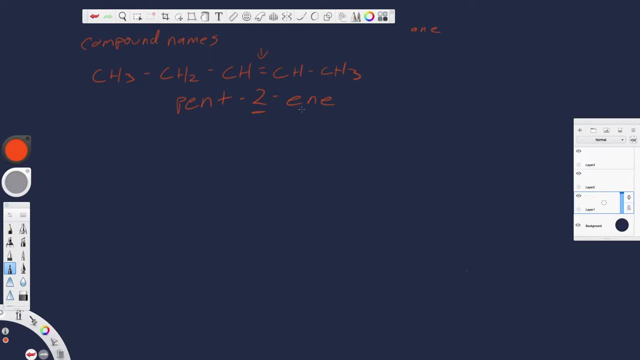 group and then the second bonding group. that's why we have this two here: two in representing the double bond and pent, of course, meaning there's five carbon groups here. okay, so that's hopefully pretty simple, pretty straightforward. in our next one we're going to mix it up a little. 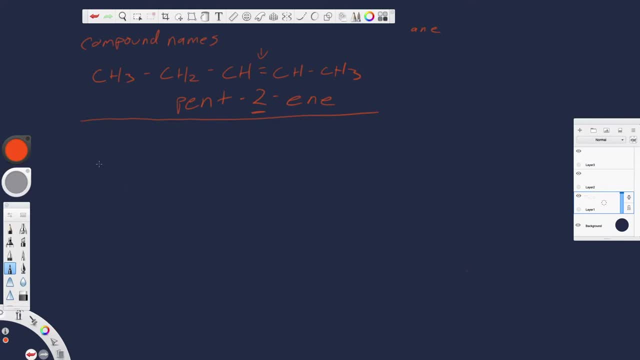 bit and add some, some branching groups here, some branching chains, and then we're going to add some chains, but still pretty, you know, not terribly complicated. but we'll say: we have a methyl group here and a methyl group here and again a double bond here on the near the. I guess you could say: 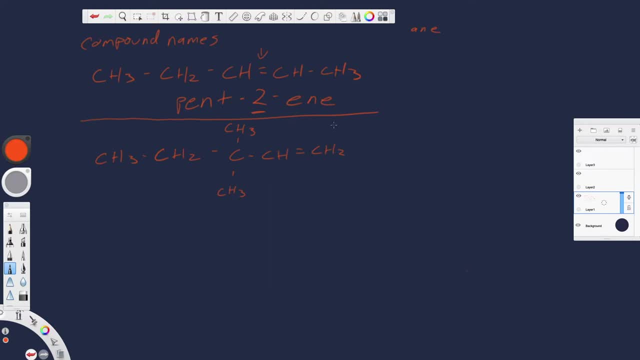 end or front would probably be more correct. uh, so now we have to be a little bit more careful about where our double chain or where our longest chain is going to be, and then we're going to add some more branches and start with this one and we're going to mark where our longest chain is. so if we 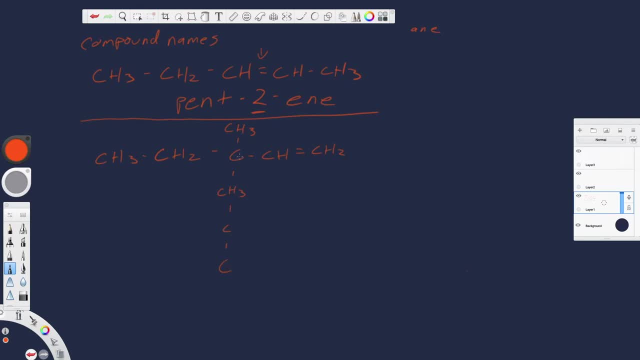 had something like this: one, two, three, four, five, six, this would be our longest chain, and in that case we would have some kind of hex like hexene, or in this case, you know, you'd have some branching chains, uh to to account. for there we go. so, but since this is our longest chain, this again is a very small branching chain. 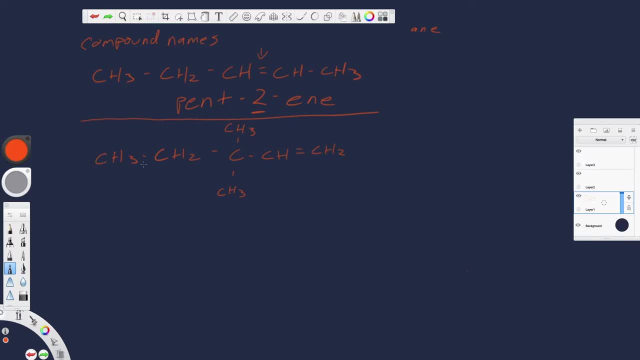 we're going to add another branching chain and this one is just going to be our longest chain is a pent. you know it would be a pentane if there's an alkane, but we have a double bond on this side. so in referencing these methyl groups, we are 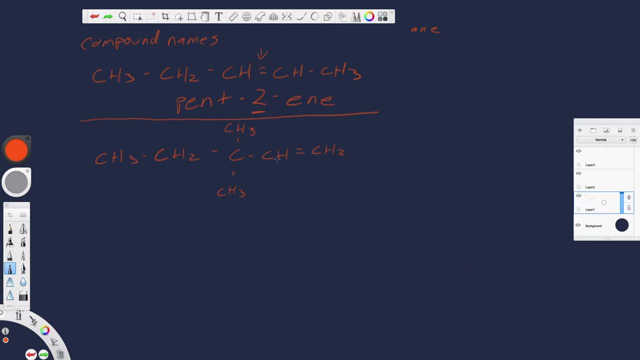 going to count from the same side as the double bond, so we're gonna have one, two, three. of course, in this case it's in the middle. so you know, happens to not matter specifically on this compound, but the correct way is to go from the side of. 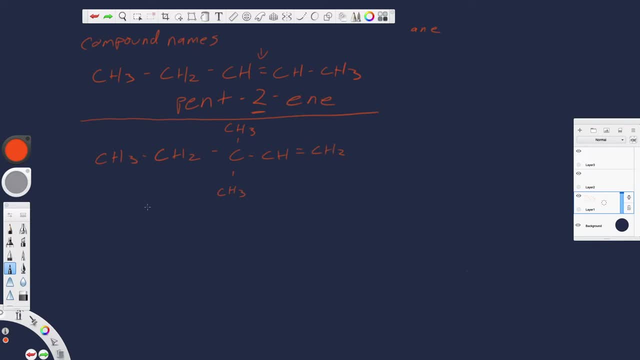 the double bond here, and so we would write this, as we're gonna start with our chains. right, we have one chain, we have a second chain, so die for our two chains at location three, three. these are methyl groups and this is a pent and it's a. 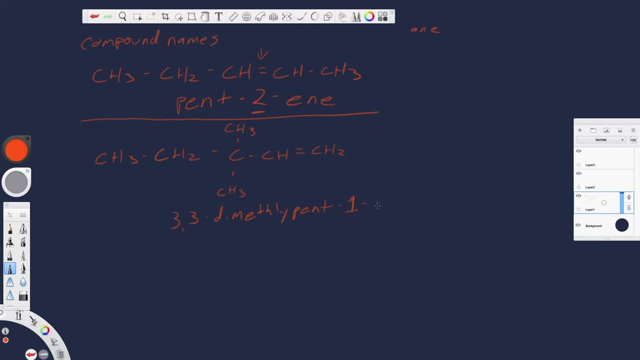 pentene located at location one. okay, so hopefully that makes sense. they all follow. you know, the simpler molecules like these all follow that same sort of convention. I mean, obviously there is a method to it. so if you can understand those basic rules you should be able to wing it through most of what is going to show up on the FE. I would. 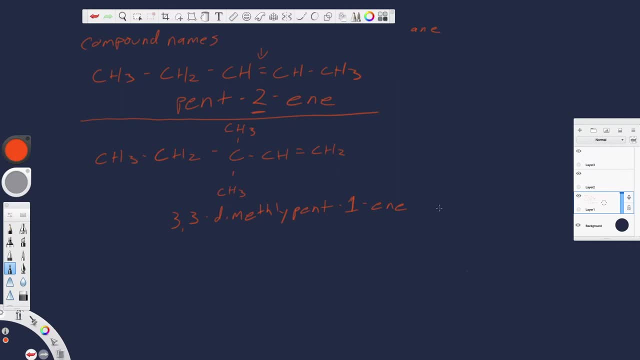 expect. I mean, it should get you covered through a lot of it, at least in the basic naming. but let's look at. another thing to kind of be on the watch out for is isomers. whoops, which is not the same as an isotope, right, an isotope has to do with. 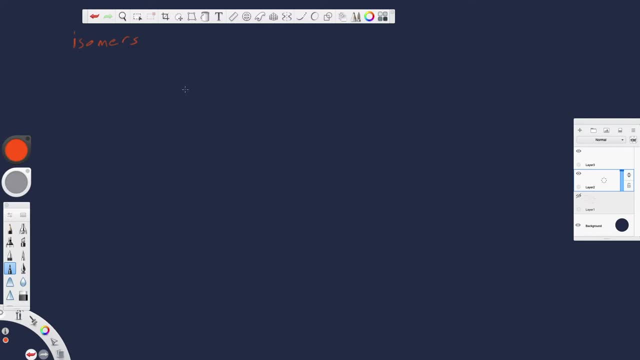 basically your number of neutrons in the nucleus of an atom. if it's they have different neutron numbers, then they have. you have isotopes. in this case it's kind of similar but you have different parts. isomers means parts. you have different parts, but a, an isomer, two compounds that. 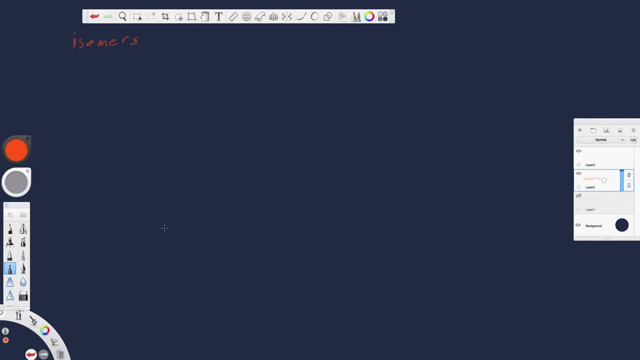 have exactly the same chemical formula been in a different structure, so you have an isomer. but it is kind of sometimes a little bit tricky. it can be a little bit tricky. you have to kind of think about what you're looking at. it may not be obvious. so, for an example, these two compounds: are they isomers? 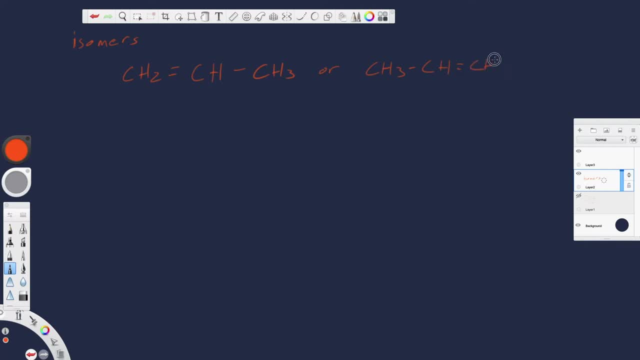 and neutrons. this is from the irritant of the Radio Worm. lets say I can see that and I can't see them. I can eat and get a little bit thirsty and then I can throw up and not have any more расcaldt nova areailos and then I say that it's. 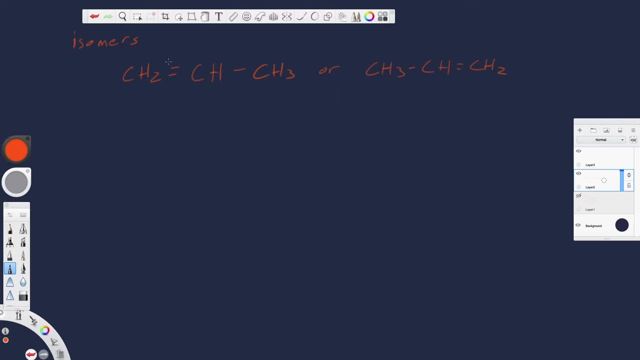 excellent. now group level two is an isomer, and what's going to be that? next thing is it's going to be the reverseート with relative frequency. and level three is a liquid atom. so this, this is the easiest possible answer, and I want you to keep an eye out for it. maybe draw some points if you overtex your takings. 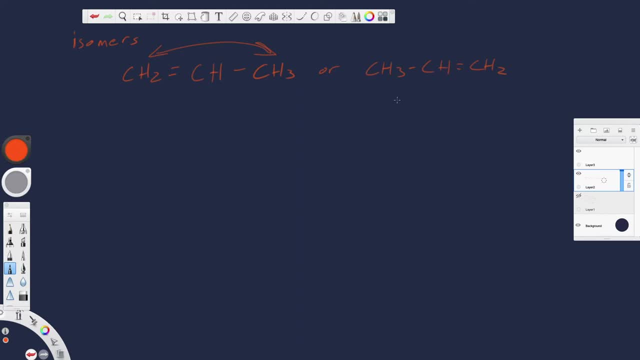 the same molecule, right, so this is not an isomer. this is the same molecule. it's structurally the same and chemically the same, um. so but what if we looked at something like um. and we're going to actually spoiler alert here, we're going to talk more about halogens, but we're also going 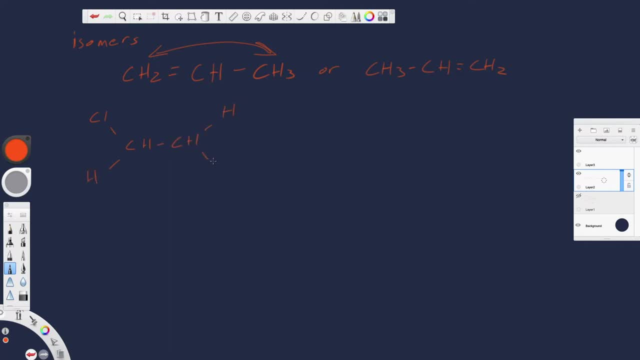 to look at them in terms of isomers, because this is one that you might see. well, i keep doing that, okay? so obviously, these are rotated or they're swapped right between each other. now, is that an isomer? and in this case, it is not an isomer, because this is a single bond. 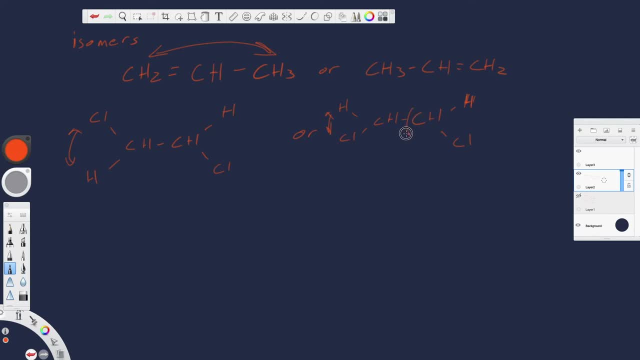 and in single bonds. these bonds are actually free to rotate, so they can rotate. you know, this side can rotate around this side, right, they can just sit there and rotate around each other. so there's no fixed structure here. so there's nothing to separate one molecule from the other. these are functionally identical. now where this might get trickier is 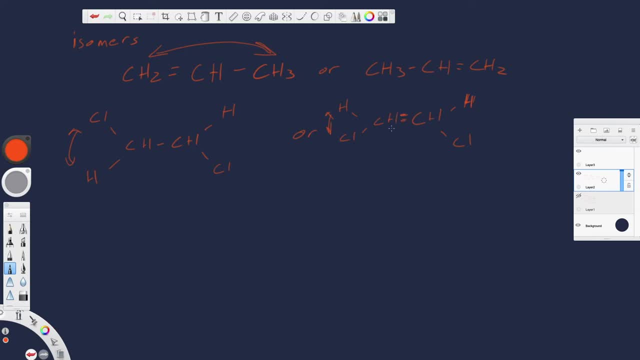 if you had- and i know this is not, it kind of messes up the chemical formula here because we have too many hydrogens- but if these were double bonds, then- and actually that's going to kind of bug me, so i'm just going to erase those. um, so if we had this: 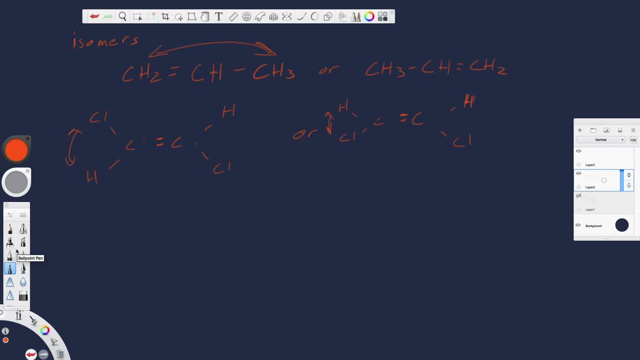 now we have isomers, because once you have a double bond, this rotation is restrained you it is difficult enough for these to rotate that these would be considered structurally different. okay, so those are a couple things to watch out for in terms of isomers and also, you know, making sure that the way that chain's branch 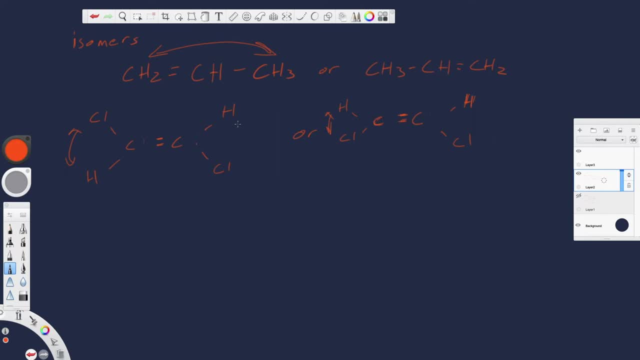 is doesn't just look different, it actually is different. right, um, okay, so the other last thing that i was going to cover- whoa, running out of time actually- is, uh, halogens, like we talked about. so your most common halogen. there we go, your most common halogen. 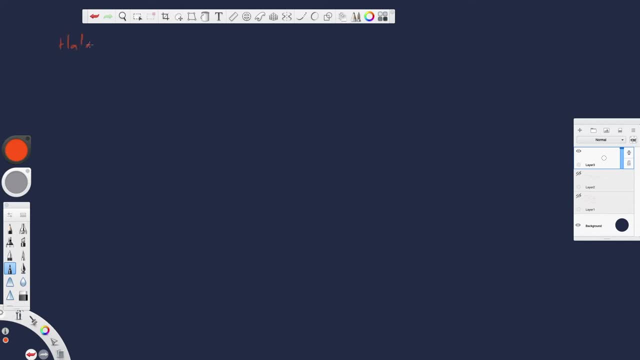 what am i? oh, i'm on the wrong. one is going to be a chlorinated halogen, and so you may have probably in your classes you've probably heard of trihalomethanes, where organic, dissolved organic matter in surface water when it goes through a drinking water treatment plant and they add chlorine, they wind up chlorinating. 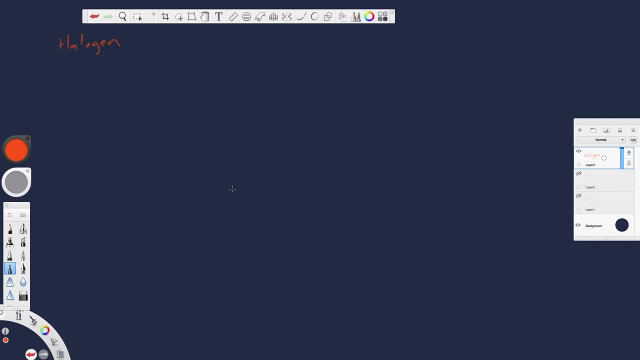 some of this organic matter and they wind up with trihalomethanes and it's a big concern in the environmental engineering industry because it's actually not really good for you to drink those. So we're looking at ways to reduce that, But anyway. so what that is is when you have 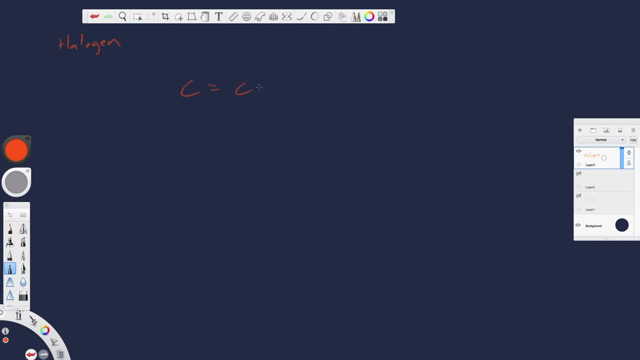 We'll look at a case. We'll look at basically the same molecule. actually, When you have That's actually Let's kind of start maybe from something a little simpler or less halogenated. at least I can't believe I did that. 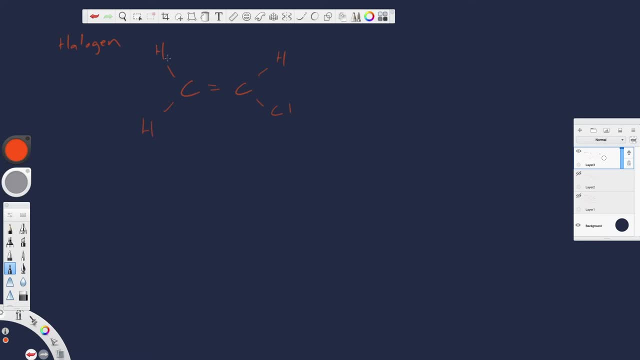 Okay, In this case this would be vinyl chloride. You've had one hydrogen replaced by a halogen, In this case chlorine, And you know that can continue to happen where chlorine comes in and basically knocks that hydrogen off and replaces it. 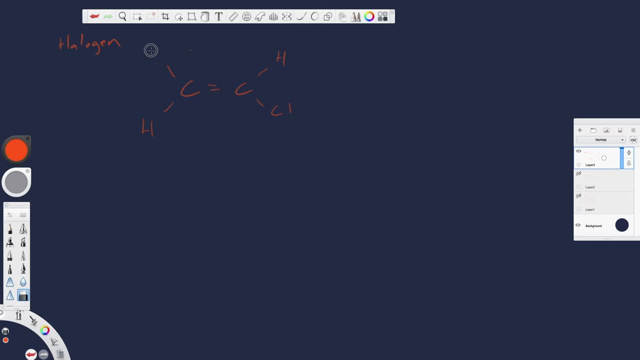 So once you have done that, or you know nature has done that, in this case you're going to have dichloroethylene or dichloroethylene. They're the same thing, It's just Different way of pronouncing it. 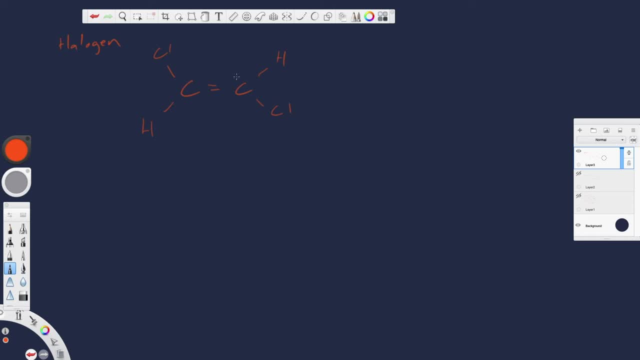 And in this case, because we talked about different isomers, this is what's called trans Transdichloroethylene, And you can also have Whoops H. This would be cisdichloroethylene. You know, because these are. 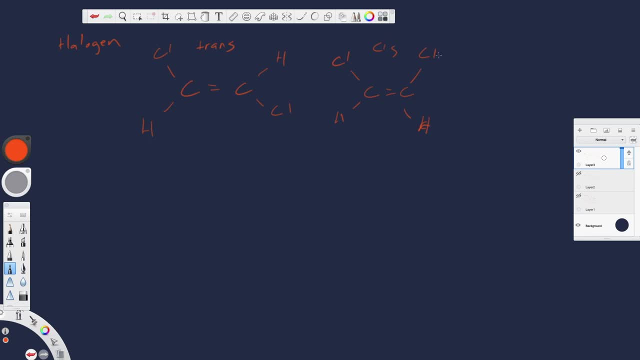 These are locked and unable to rotate. the orientation of the halogens makes a difference, right, And if they're on the same side they're cis molecules or halogens. If they're opposite of each other within the same plane, then they would be trans. 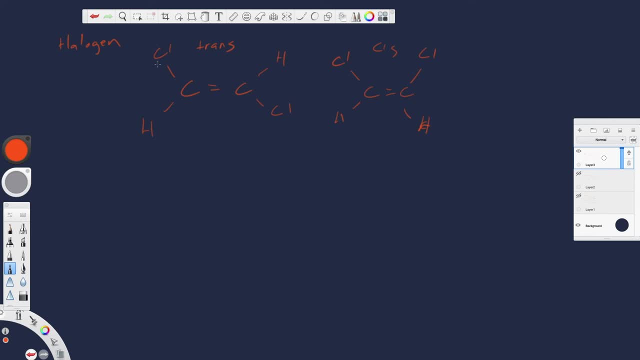 And that also It's not just halogens, That's basically organic chemistry in general follows that rule, that naming convention. So that's one other thing to You know, be aware of, And the only other thing I guess to maybe mention before we call it a day on this episode. 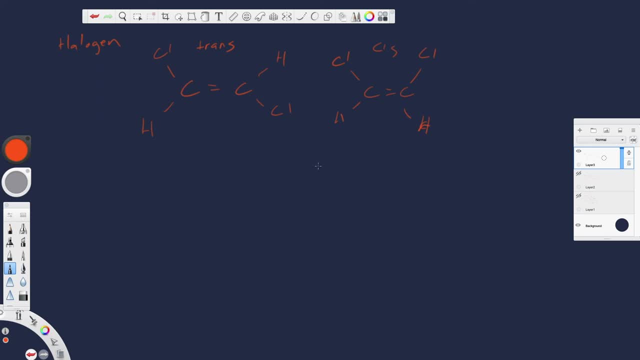 is to just be aware of your functional groups. It might, You might be asked about identifying a functional group, or what is the functional group, or you know what's the most important aspect of an organic compound? It's going to be your functional group. 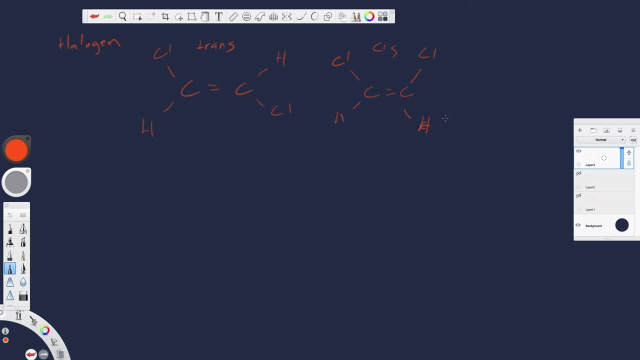 And that's where, basically, you just have these things that You know, these groups that attach to the organic molecule like a hydroxide, which would be an alcohol, right? So if you had like C, C and then hydrogen hydroxide, I mean. 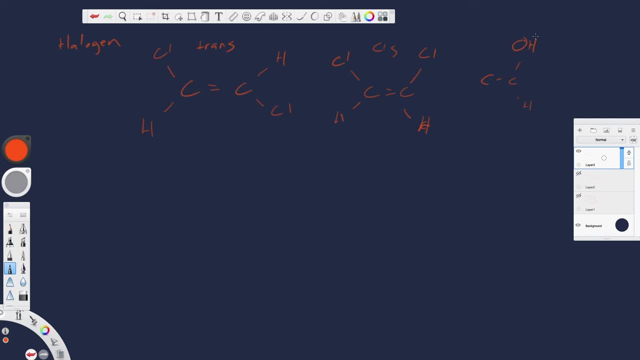 this would be ethanol, right. So this functional group changes the molecule in a very meaningful way And it really kind of defines how that The properties of that molecule, like methane or methanol and ethanol, are going to be somewhat, fairly, quite similar really.